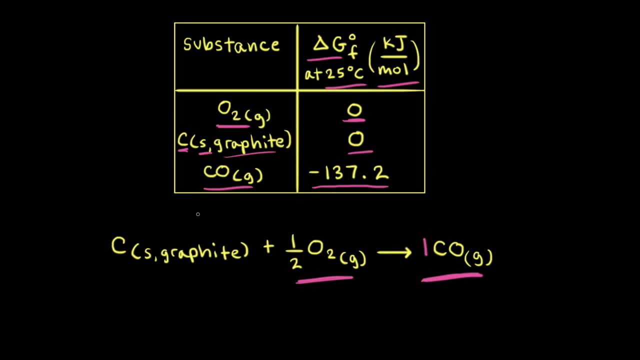 And the elemental form of oxygen is O2 gas and the elemental form of carbon is the solid form in graphite. So this value for the standard change in free energy of formation of carbon monoxide is talking about the, the change in free energy for the formation. 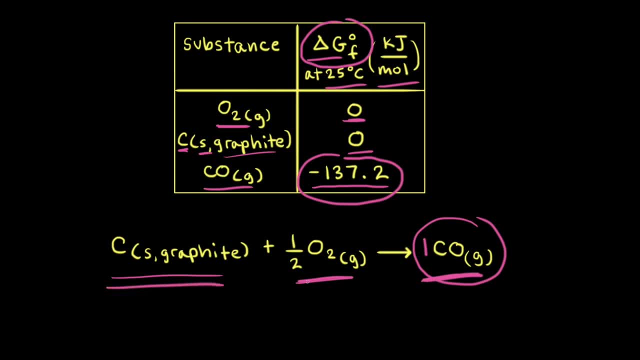 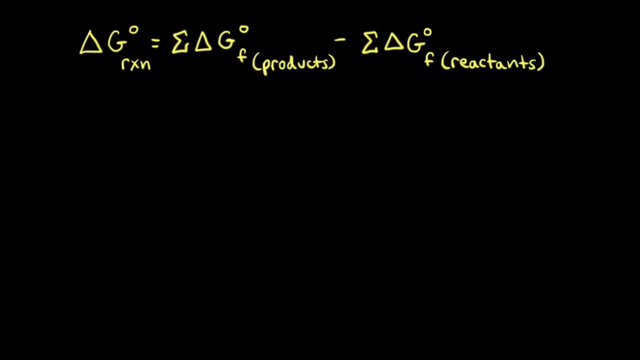 of one mole of carbon monoxide from its elements in their standard states. Standard changes in free energy of formation of substances are useful because they can be used to calculate the standard change in free energy for a chemical reaction. The standard change in free energy of a chemical reaction. 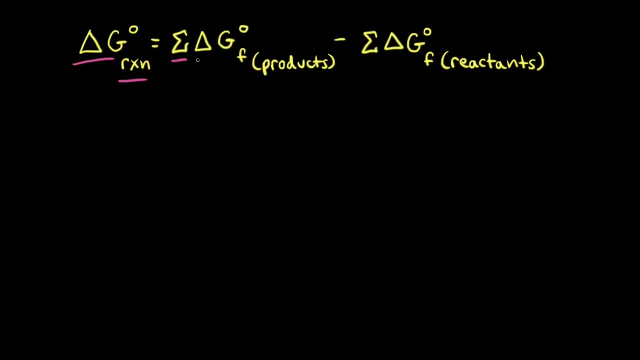 is equal to the sum of the standard change in free energy of formation of the products, And from that you subtract the sum of the standard change in free energy of formation of the reactants. For our reaction, let's look at the synthesis of ammonia gas. 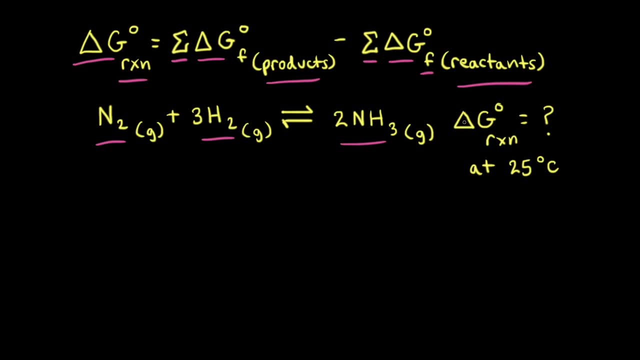 from nitrogen gas and hydrogen gas. Our goal is to calculate the standard change in free energy for this reaction at 25 degrees Celsius. First we need to think about our products. For this reaction we have only one product, and that's ammonia. 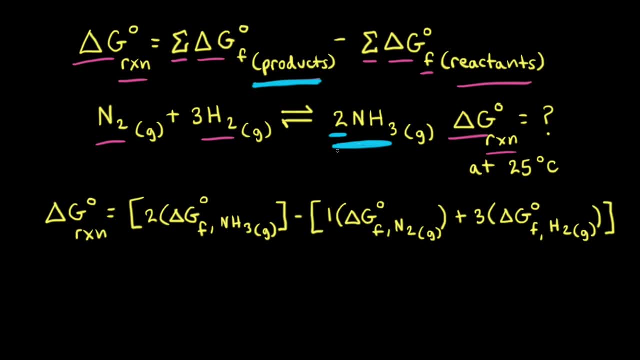 Notice how there's a two as a coefficient in front of ammonia in the balanced equation. So we would need to look up the standard change in free energy of formation of ammonia at 25 degrees Celsius And because this value is per mole of ammonia. 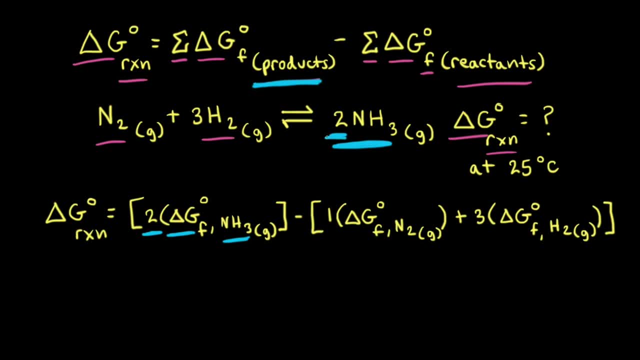 we would need to multiply it by two, because we have two moles in our balanced equation. Next we think about our reactants, and we have two reactants, nitrogen and hydrogen, And we need the sum of their standard changes in free energy of formation. 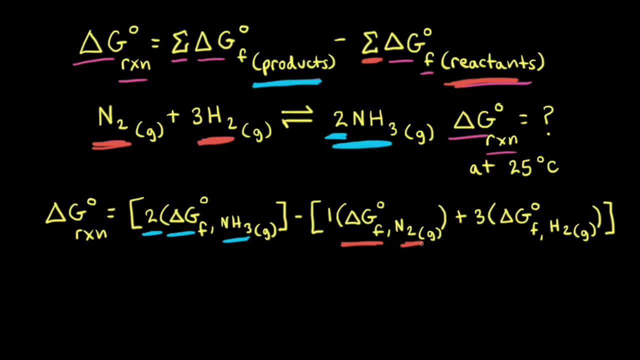 So we would write the standard change in free energy of formation of nitrogen, And because there's a one in our balanced equation, we multiply that value by two, We multiply that value by one, And to that we add the standard change in free energy of formation of hydrogen gas. 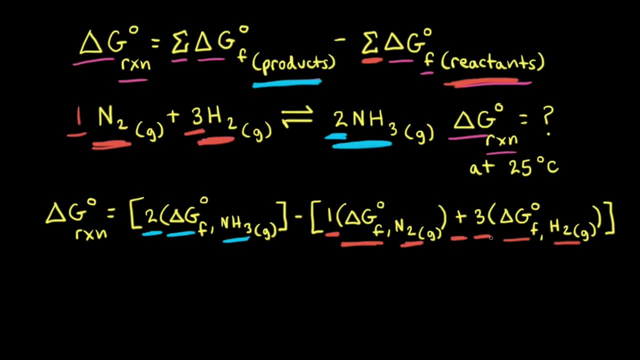 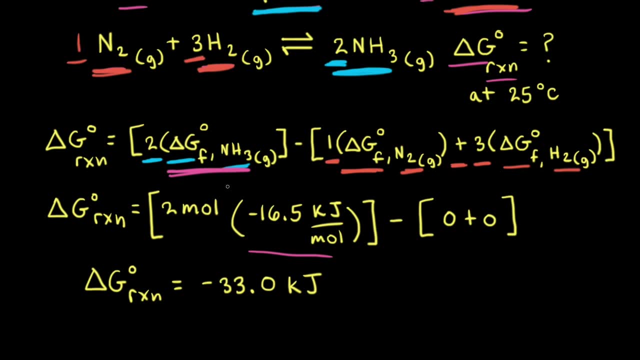 And since we have a three in our balanced equation, we would multiply that by three. So, going back to ammonia, the standard change in free energy of formation is equal to negative 16.5 kilojoules per mole. Multiply that by two moles and the moles will cancel out.